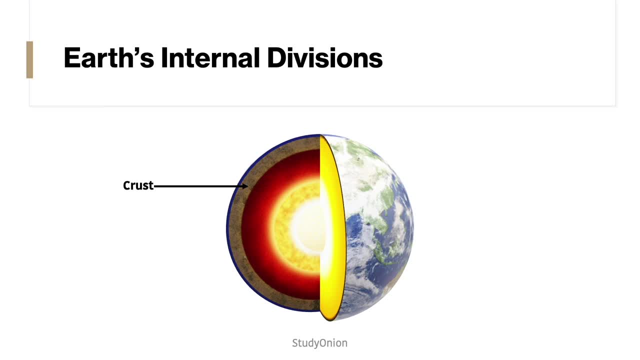 There are two different types of crust: continental and oceanic crust. Older continental crust consists of low density rocks such as granite, and the younger and thinner oceanic crust contains darker and denser rocks such as basalt. The most common elements in the crust are silicon and oxygen. 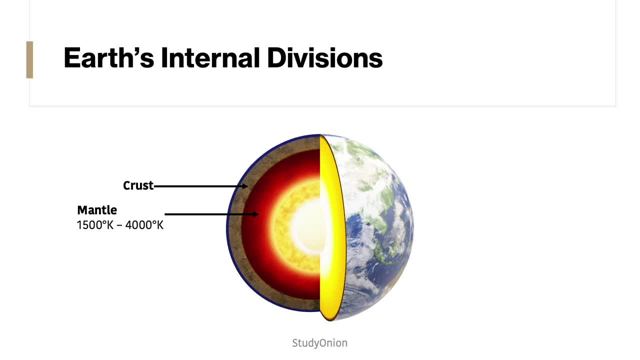 After the crust. the crust is made of silicon and oxygen. After the crust comes the mantle. This is a silicate shell which has a thickness of around 2,900 kilometres, making up around 80% of the Earth's volume. The lower mantle, also known as the asthenosphere, is solid. 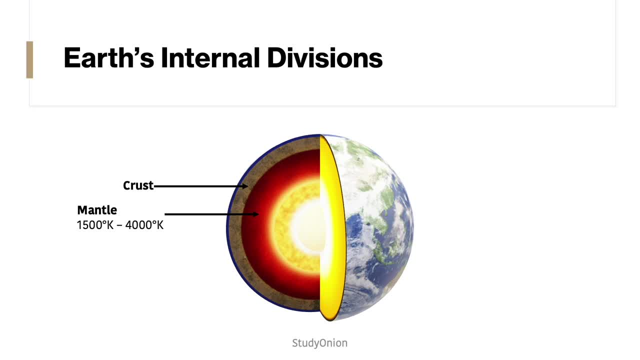 Whereas the upper mantle, or lithosphere, is semi-molten, which allows these convection currents to rise and fall, driving the motion of the tectonic plates. The outer core is a liquid layer of iron and nickel. It is about 2,266 kilometres thick and has a temperature of around 5,000 kelvin. 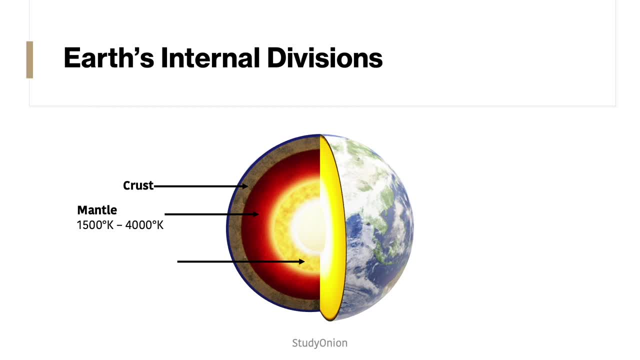 The charged particles which flow in here are responsible for the Earth's magnetic field, which protects us from the radiation that comes from the Sun. The inner core, which is at temperatures of around 5,500 kelvin, prevents the iron and nickel and prevents the atmosphere from melting. 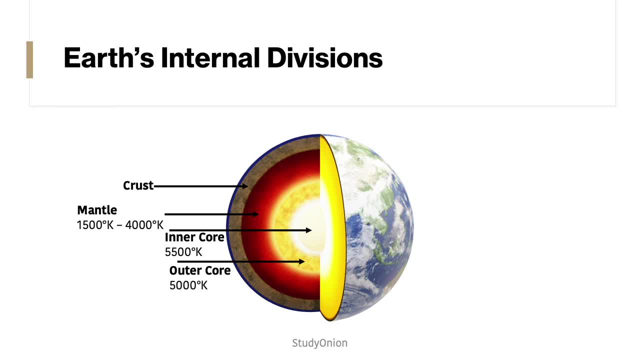 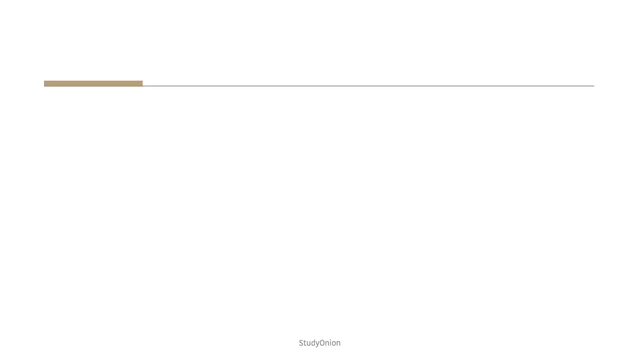 Moving on to talk a little bit more about the atmosphere. The Earth also beholds a rich atmosphere of nitrogen and oxygen, and most of the Earth's surface is actually covered by oceans of seawater. Now let's have a little look at the benefits and also the drawbacks. 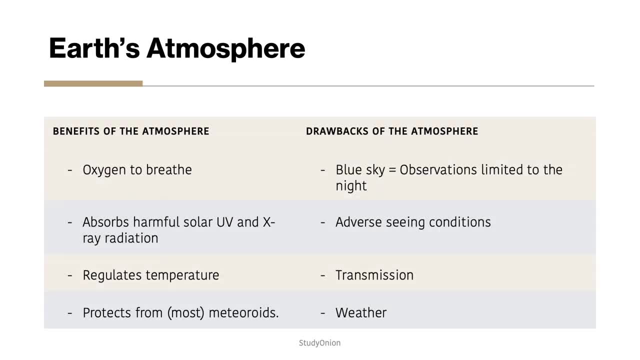 of the atmosphere. The atmosphere has many, many benefits for us: Oxygen, which allows animals and plants to breathe. Carbon dioxide, allowing for photosynthesis. It makes the climate and temperature of the Earth consistent, of a mean of around 15 degrees Celsius. 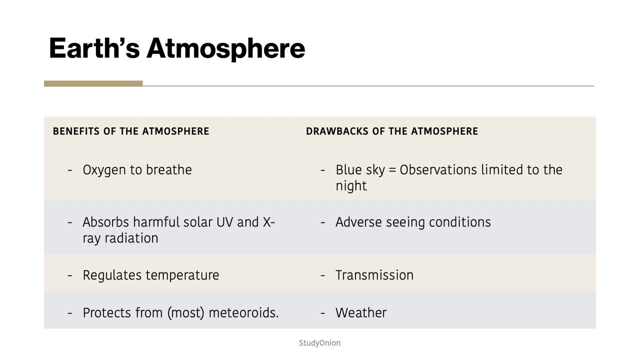 It spreads out and scatters light from the Sun, protects us from micrometeorite collisions in space and protects us from the harmful UV radiation, or ultraviolet radiation, that comes from the Sun. However, there are a few disadvantages of the atmosphere for astronomers. 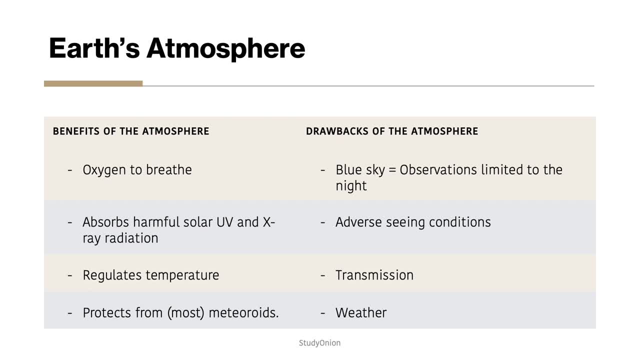 Firstly, scattering. The sky is blue, which limits observations to nighttime. Light from the Sun is scattered by these nitrogen and oxygen particles in the atmosphere And because most of this scattering occurs at these shorter wavelengths of blue and violet light, the sky is predominantly blue. 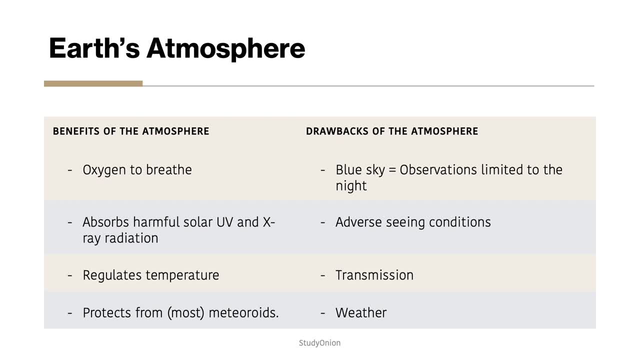 The sky can also be red at sunset, And you might wonder why this is. This is because, when the Sun gets lower in the sky, the light emitted is travelling through more of the atmosphere before it can pass through and reach you. This means more of the blue light is scattered away. 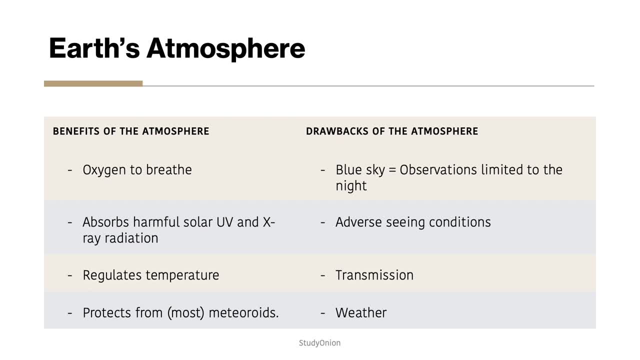 leaving only the yellow and red light left Seeing. The air in the atmosphere is continuously rising and falling. Different densities of air rise and fall at different rates, causing the light to refract and change direction as it passes through many different layers. 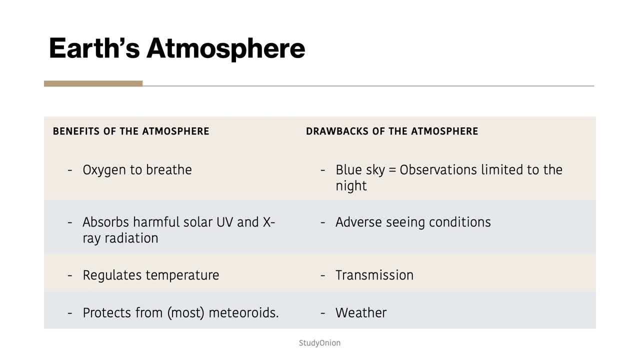 This makes the stars appear to twinkle. This is worse for stars lower near the horizon because the light must travel through more of the atmosphere Seeing conditions. These conditions can be measured using the Antoniadi scale Transmission. Many of the objects in space are only visible in parts of the EM spectrum that we cannot see. 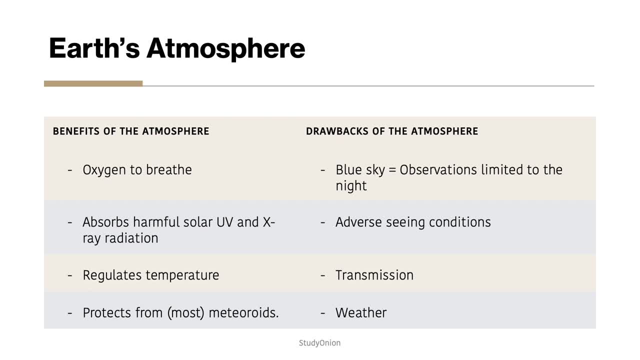 Ultraviolet and infrared, for example. The atmosphere observes many of these, and thus we cannot see them in our observations. Weather: The Earth's weather can block out our view of space By clouds, for example. Light can also be scattered by dust storms. 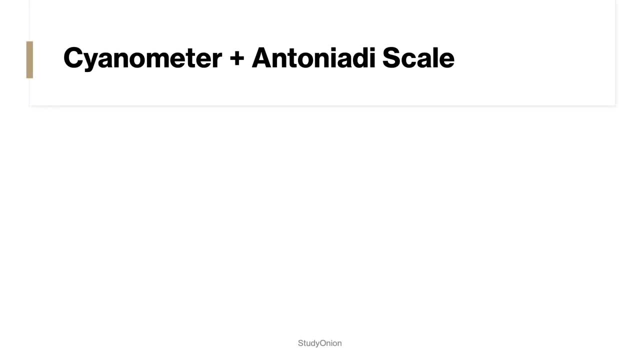 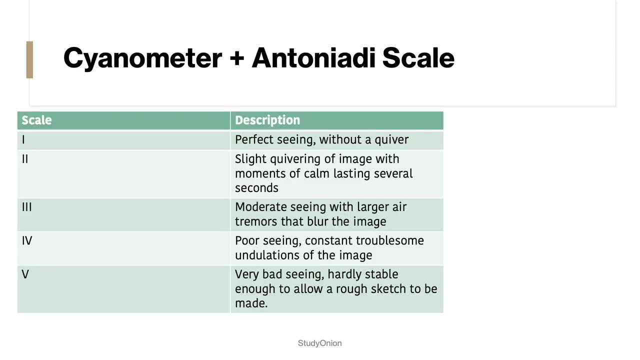 and other weather patterns. So let's have a quick look at the cyanometer and the Antoniadi scale. So this shows the Antoniadi scale, which is a scale used to measure seeing conditions, and the cyanometer is used to determine the blueness of the night sky. 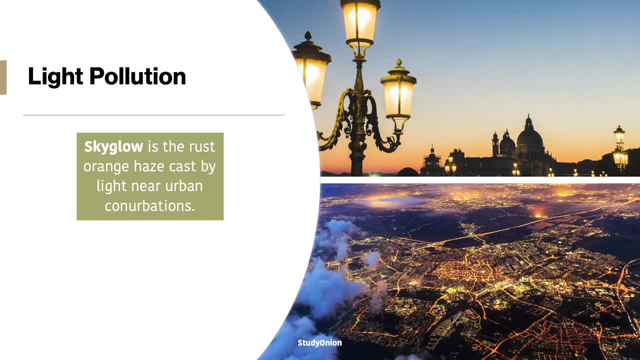 Another issue for astronomers is light pollution. The sky glow, is the rusty orange haze cast by lights near urban cities and local glare from sports grounds, supermarket, car parks, street lights and security lights that ruin the dark adaptation of their eyes. Just to clarify by dark adaptation: